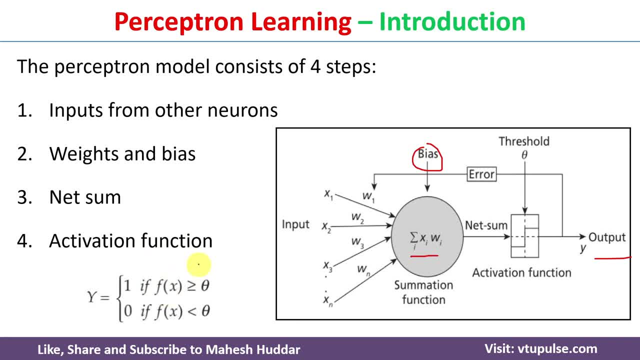 there, just for explaining, i am considering the step activation function here. in step activation function, if the calculated sum this one, if it is greater than or equivalent to some threshold value, the output will be 1. here, if it is less than some threshold value, it will be equivalent to 0. here, 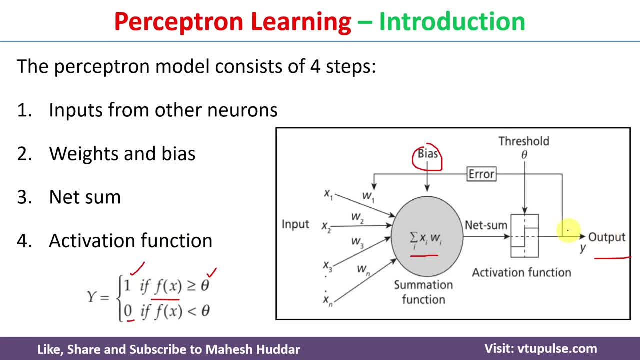 so, based on the activation function, we will get different outputs here. once you calculate the output, we will compare this output against the actual output and then we will calculate the error. and once you calculate the error, we will check whether the error is acceptable or not. if it is not, 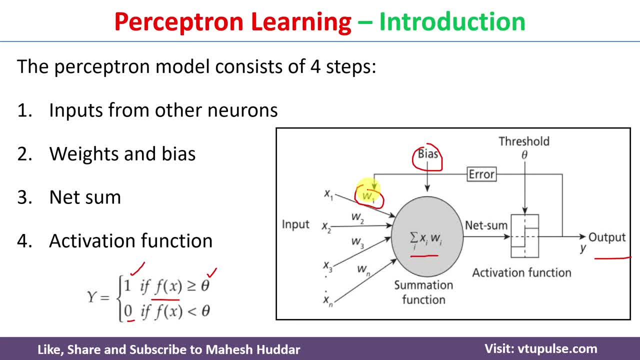 acceptable. we will update the weights in this case. so we will try to understand the perceptron learning algorithm step by step here. first, we need to initialize all these weights here for each and every input. as said earlier, there will be weights and the bias here, so we need to. 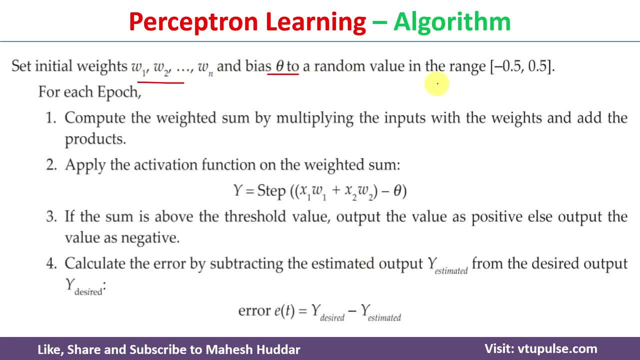 initialize these weights, as well as the bias, randomly, usually in the range of minus 0.5 to plus 0.5 here now for each epoch. until we will be able to classify each and every example correctly, we need to perform the following steps here. so in the first step we need to compute the weighted 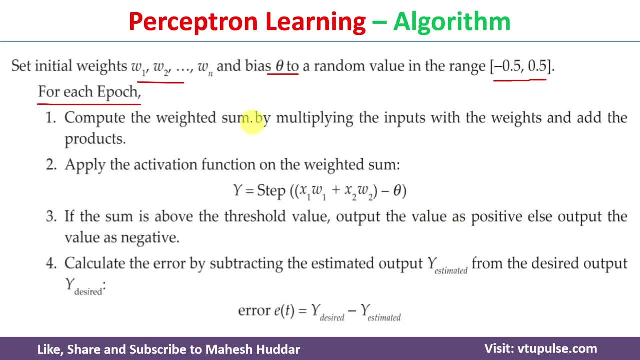 sum. as said earlier, we need to compute this weighted sum here. once you compute the weighted sum using the input and the weights, we need to apply the activation function. as said earlier, we need to apply the activation function so that we can calculate the output here. so first we will. 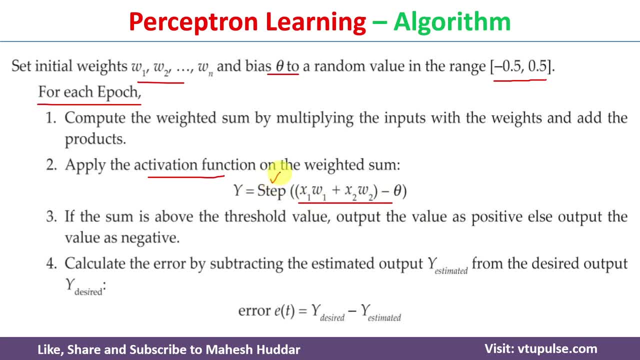 the weighted sum here. on the top of that we will apply the activation function again. just for explanation purpose, i have taken step activation function here. now, once you calculate this output, we need to calculate the error by subtracting the estimated output. estimated means the calculated output from the desired output. that is nothing but the target output here. so we have some target. so 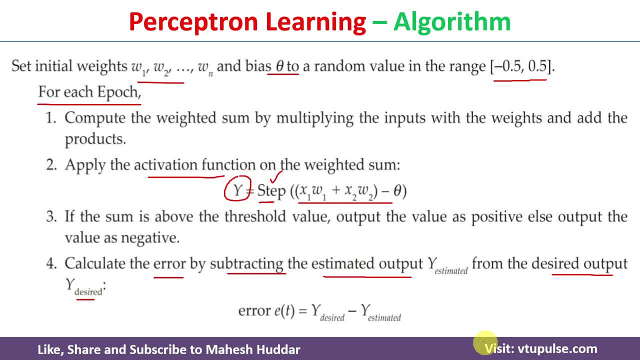 the calculated output will be subtracted from this target output so that we will be able to calculate the error here. so once you calculate this error, if we are happy with this error, there is no need to do the weight updation. if we are not happy with this error, we need to go back and update.